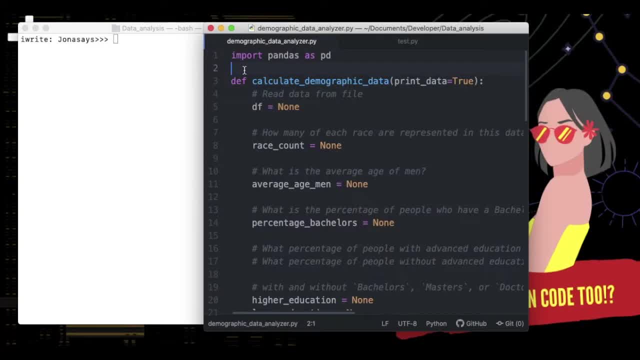 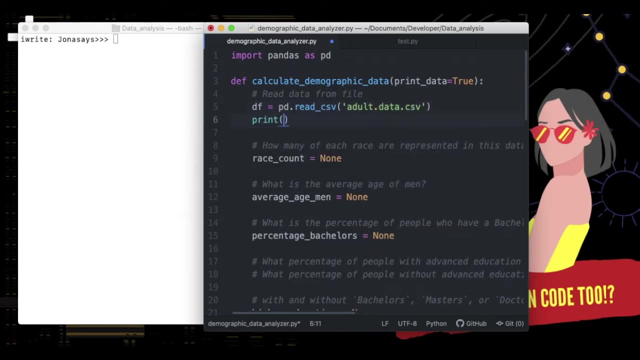 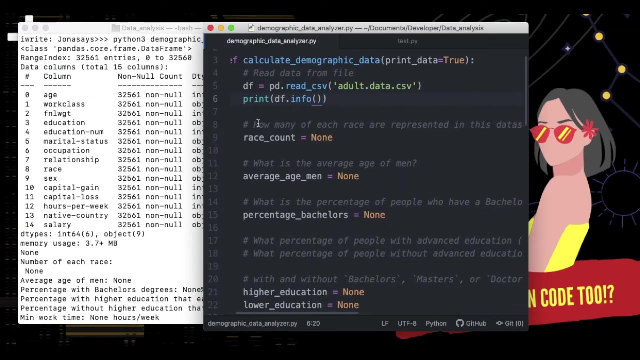 And I copy it paste to my atom. and now ready to code. First we need to read CSV file using pandas. read CSV and put file name here. Let's print info. Now it shows columns and what are inside the columns. Next they ask us to show each race in this database. 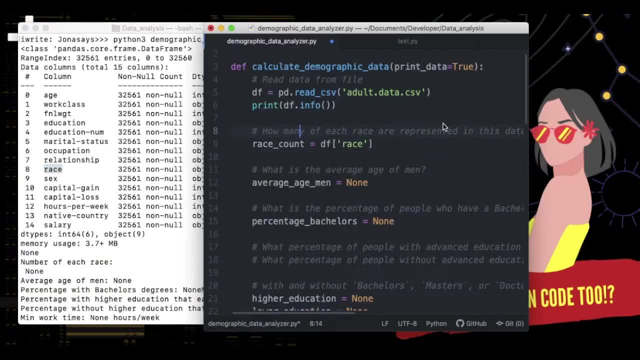 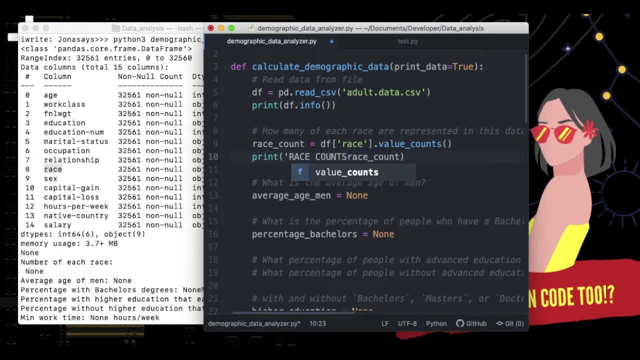 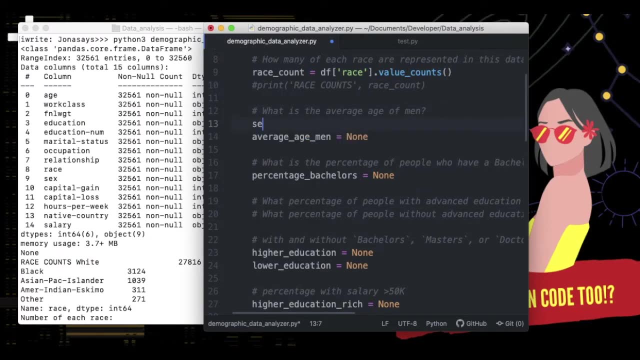 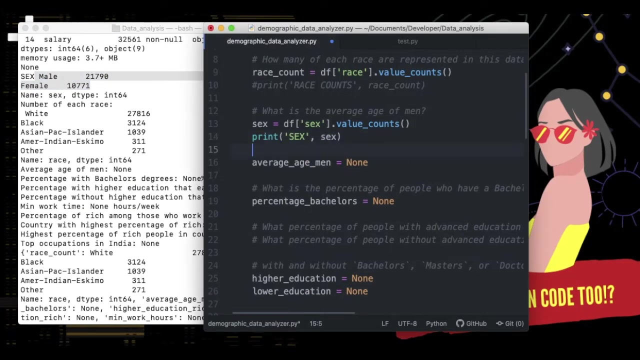 So we will select column race and use function value counts to show data in this database. Let's find this race column. Next, find an average age of men. First, show me all the gender. There are male and female. Now select gender that is only male. 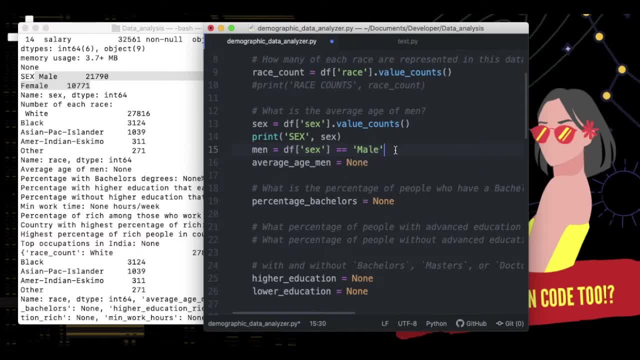 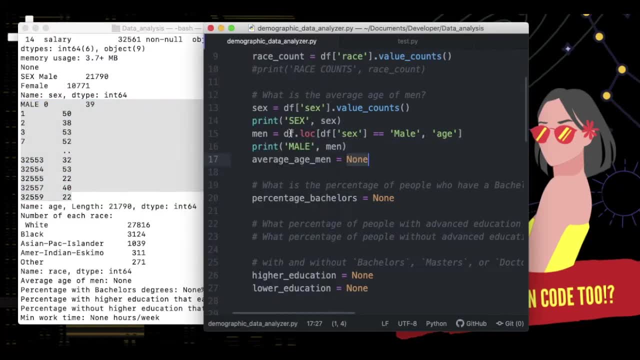 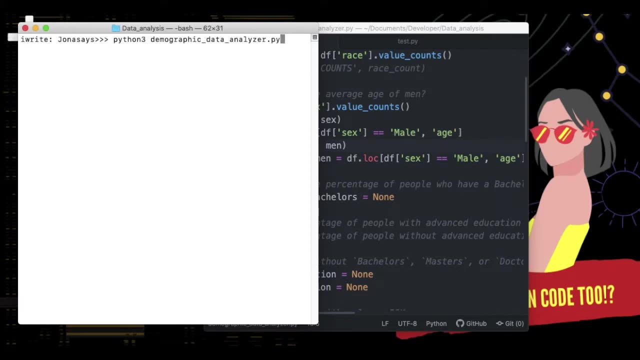 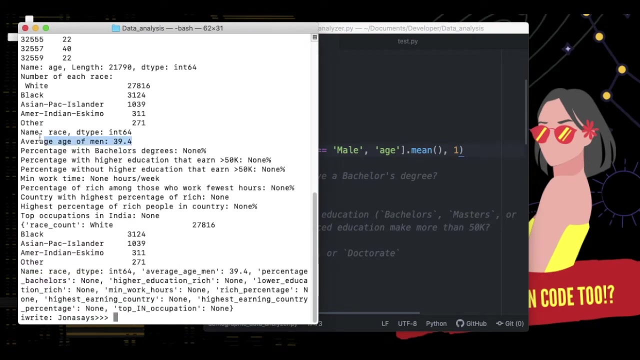 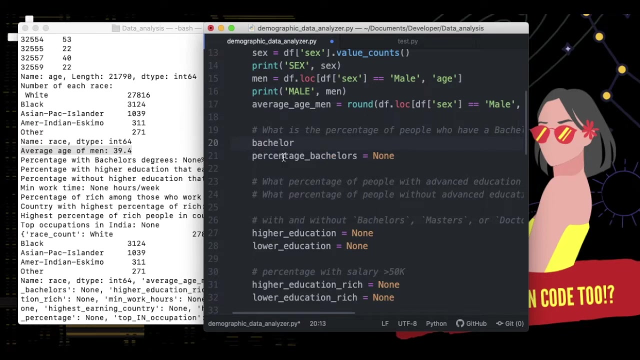 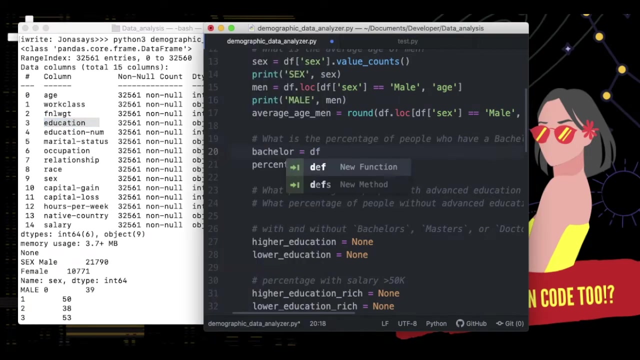 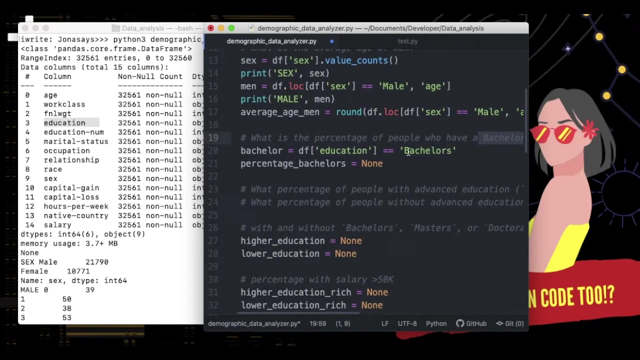 and show me age column. Then find mean. Next, find how many people who have bachelor's. First be find who have bachelor's. Select column of education. filters by bachelor's. Then click on right bottom the bar, then click on showed web and we can see that the profile page should be shown on the left hand side. 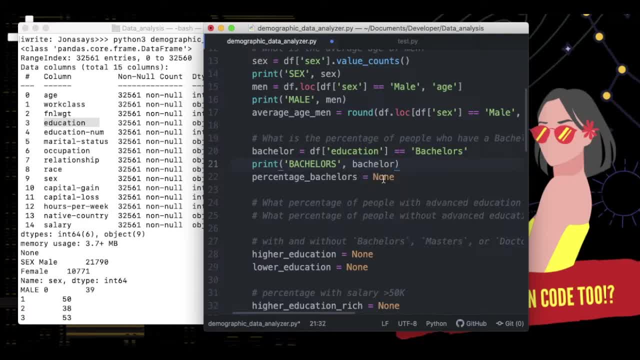 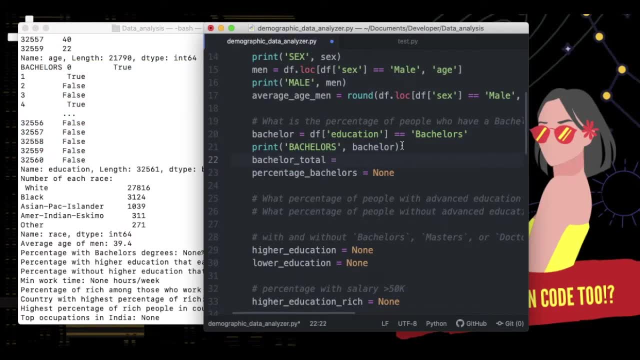 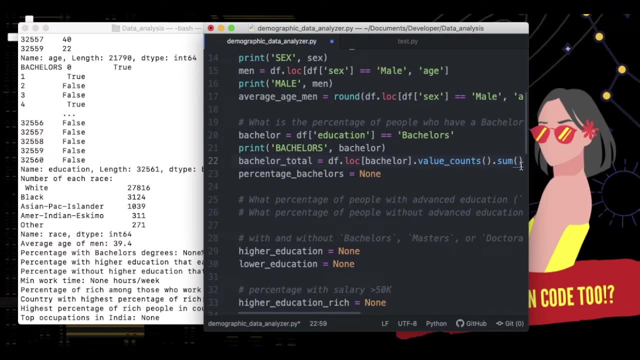 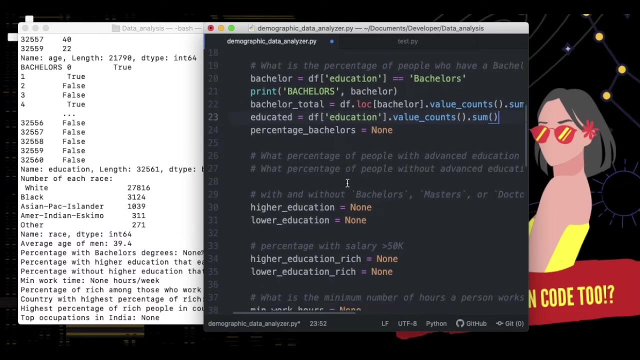 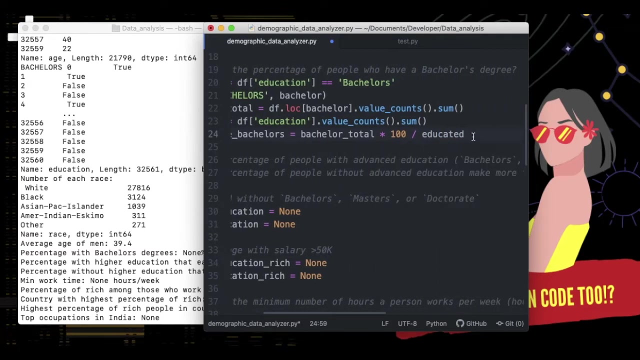 hit enter and here it's shown as shared. Let's see what is not shared. Let's see It shows only next year, or change option. Let's find substitutes here. Then we need a total number of every types of education. Then calculate percent of people who have bachelor's. 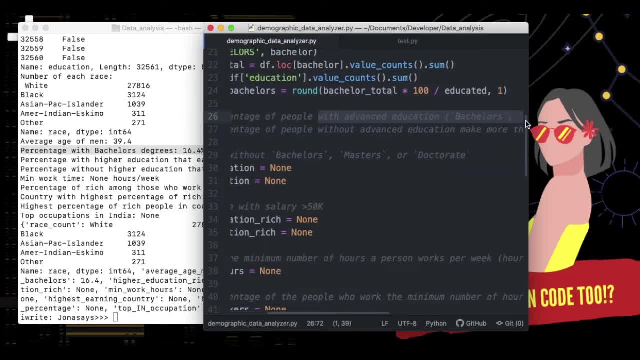 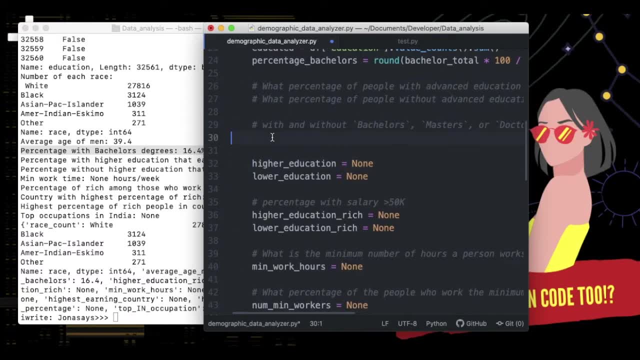 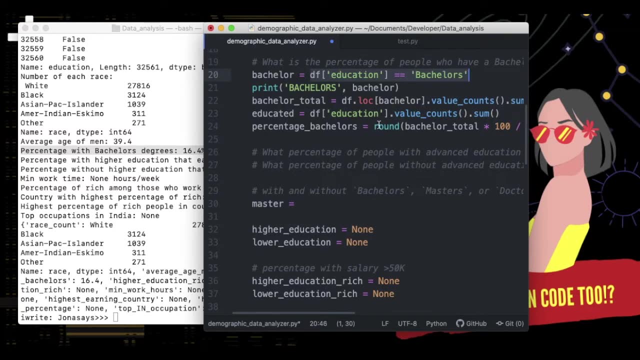 And then next 5% of people with high education and rich, And also 5% of people without high education and rich. So first we find people with high education by selecting column of education with bachelor, And then do the same with master and also doctorate. 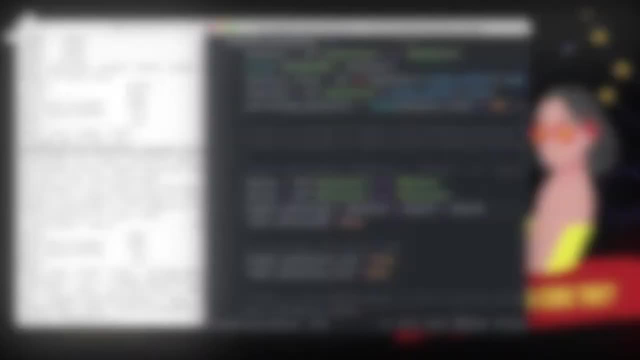 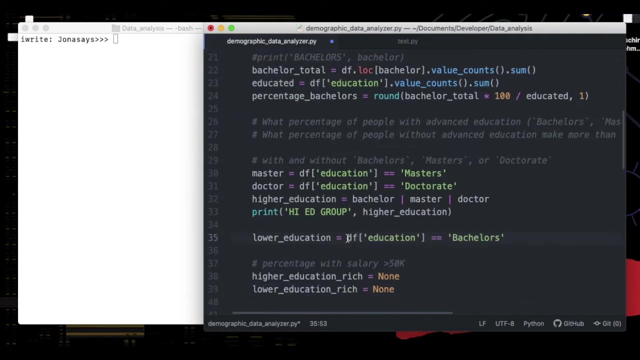 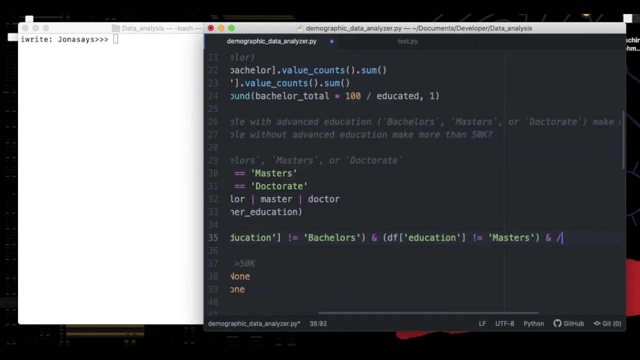 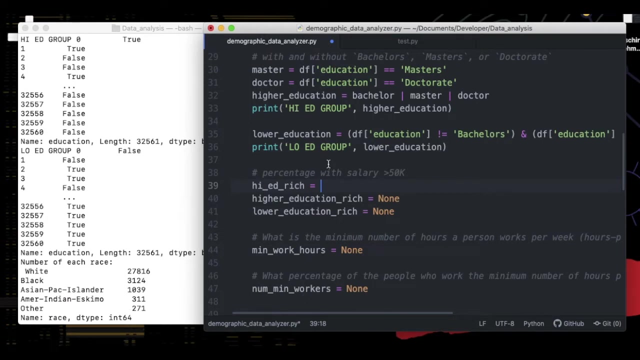 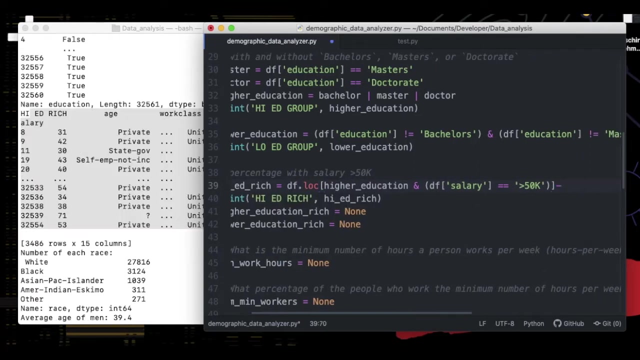 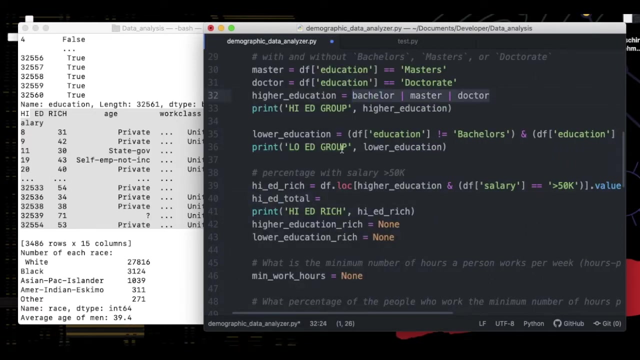 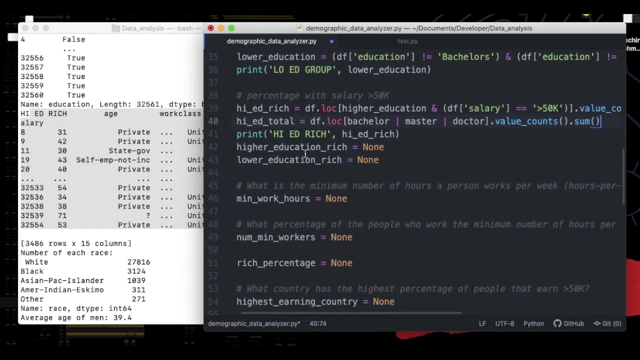 And then click off those who are without bachelor, without master and without doctorate. So to calculate percent we want a total number of high educated people who are rich And total number of high educated people. Then calculate percentage of rich people in this group. 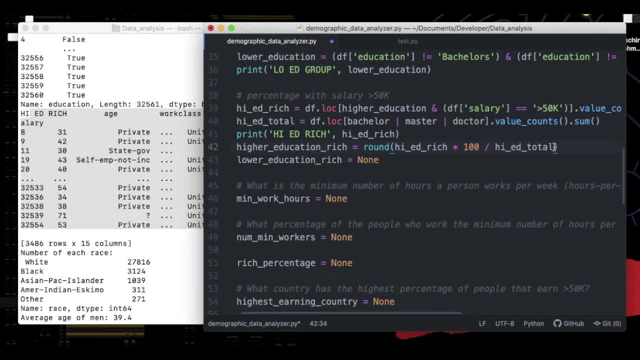 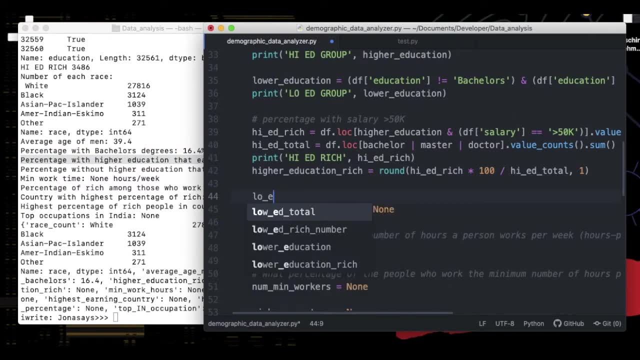 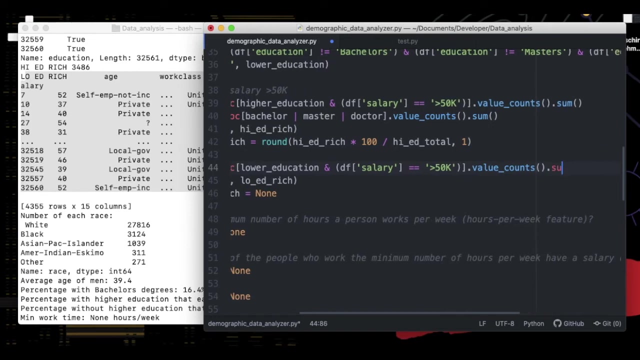 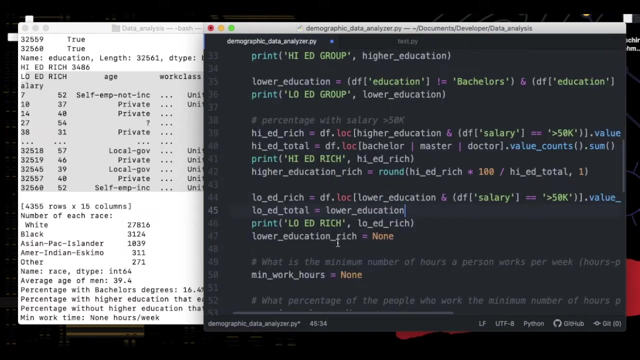 Ok, Next, do the same: that find total number of low educated people who are rich And total number of low educated people. Ok, Next, find the minimum number of hours a person works per week And calculate percentage of rich people in this group. 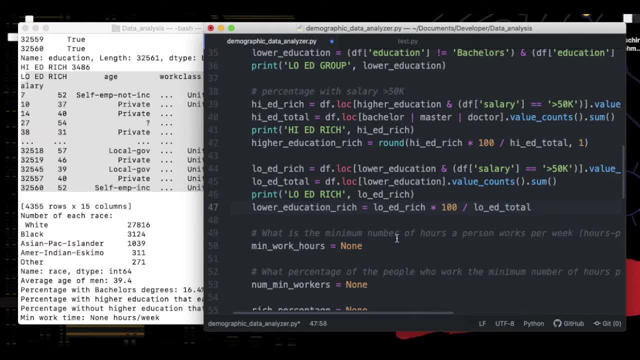 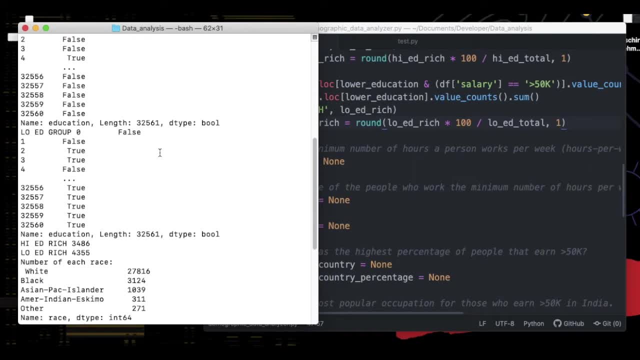 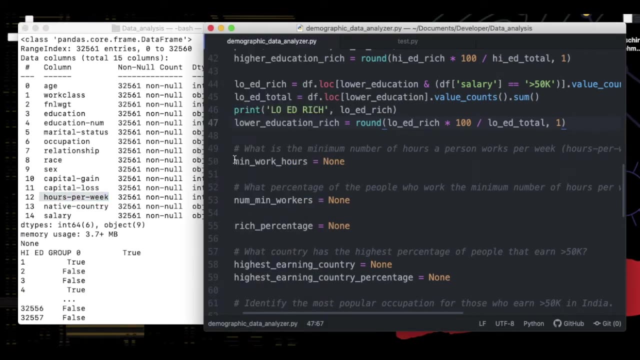 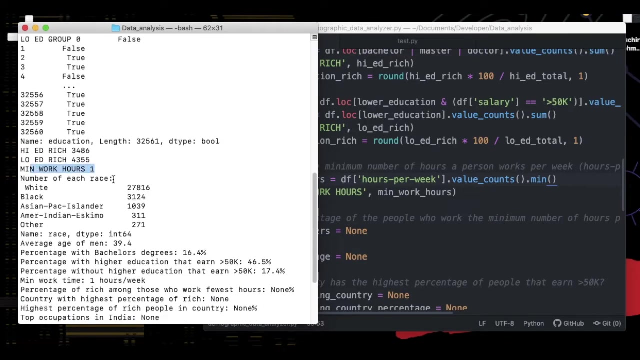 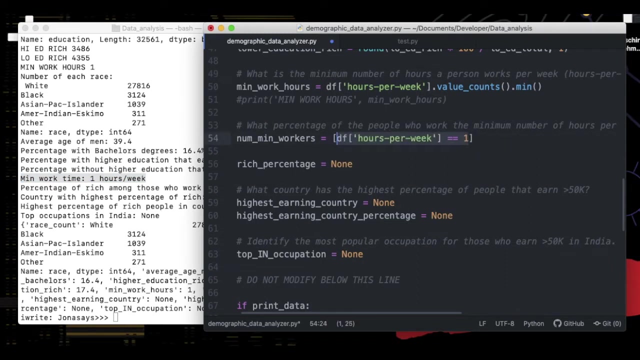 Then do the same. Next, find the minimum number of hours a person works per week. Ok, that's all of to-do list. Thanks for watching. First, select column of hours per week and then find min. Next, calculate percent of people who work minimum hours and get rich. 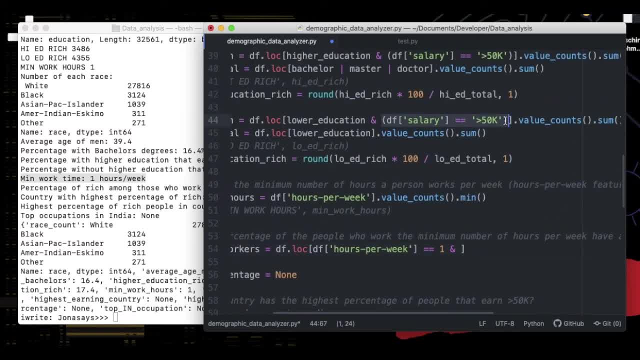 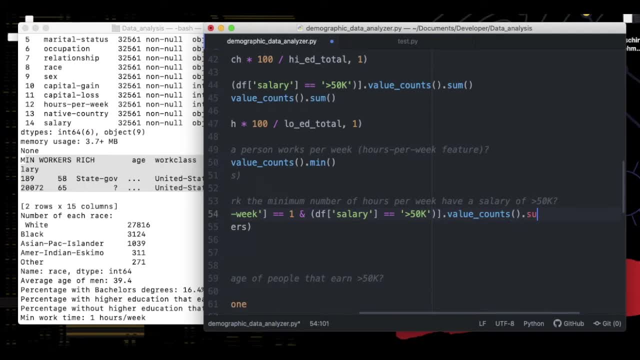 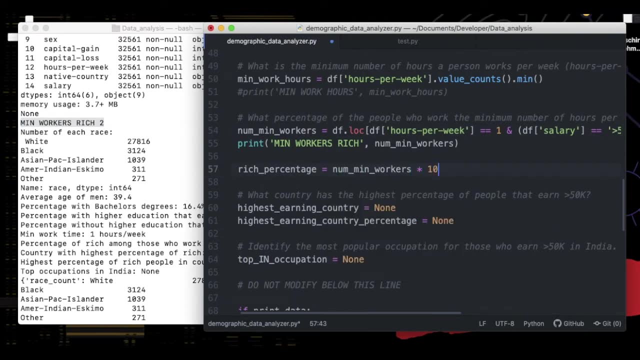 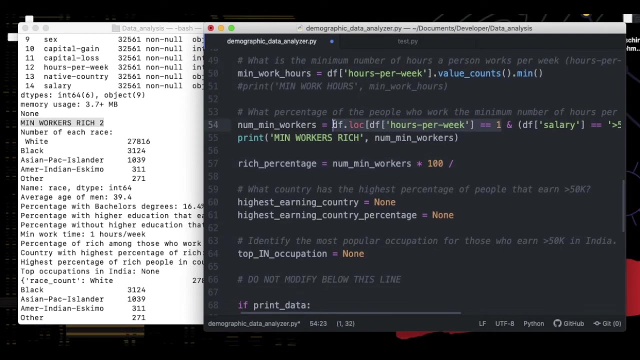 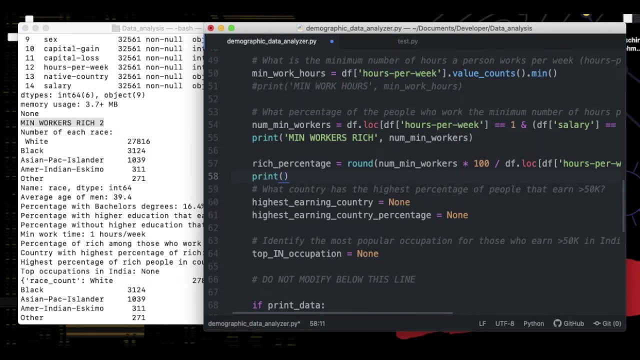 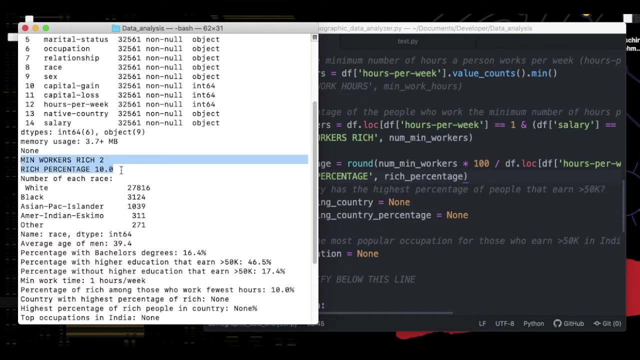 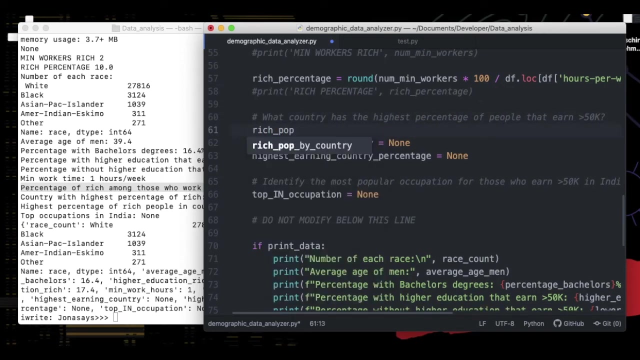 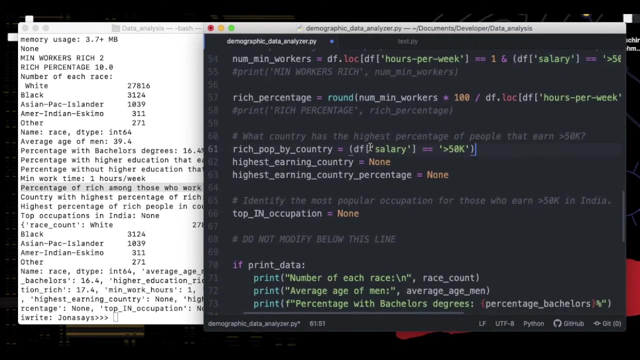 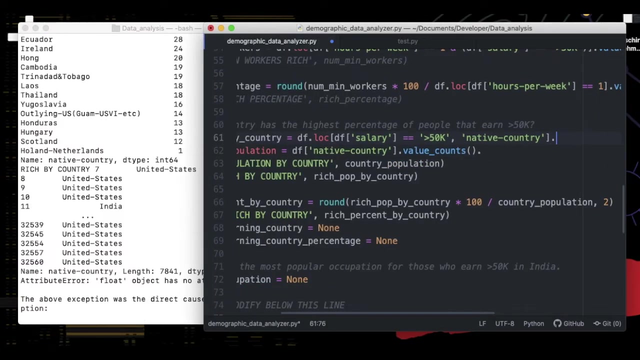 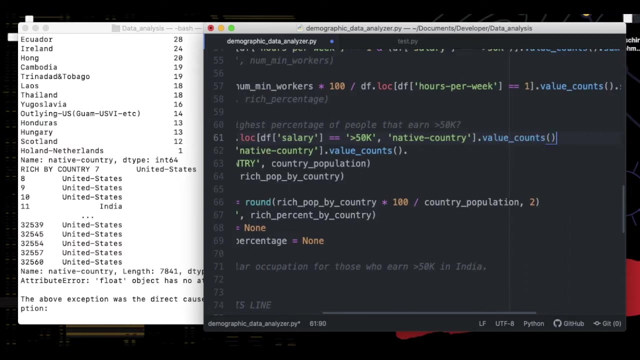 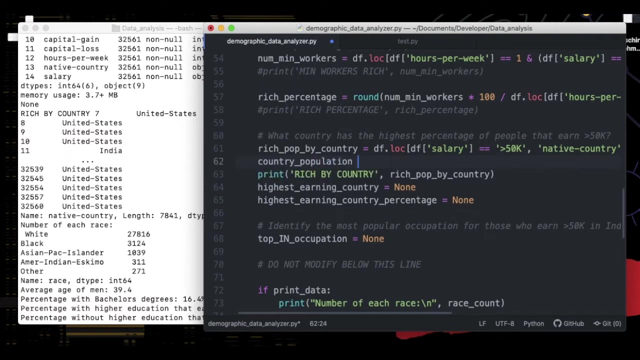 So we need to find a total number of people who work minimum hours and rich And then calculate to a percentage. Next, which country has the highest percentage of rich people? We need to find rich people and show me the country, Then find total population of each country so we can calculate percentage of the rich. 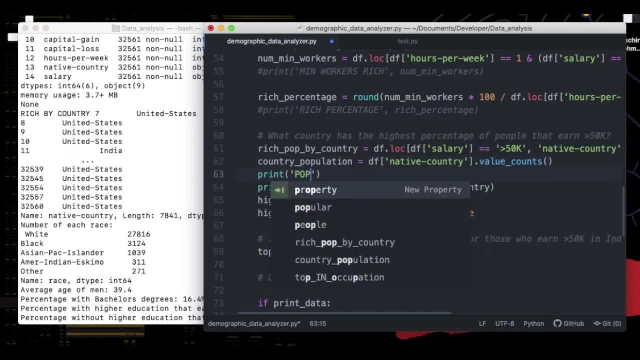 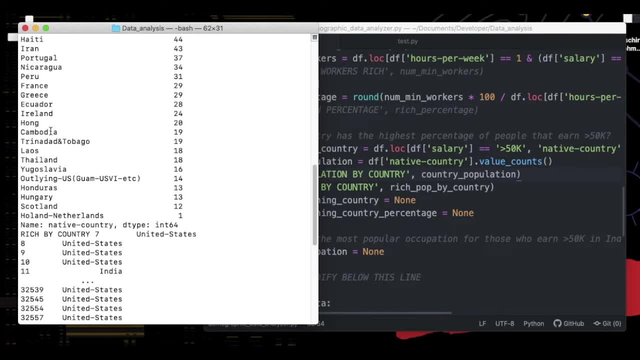 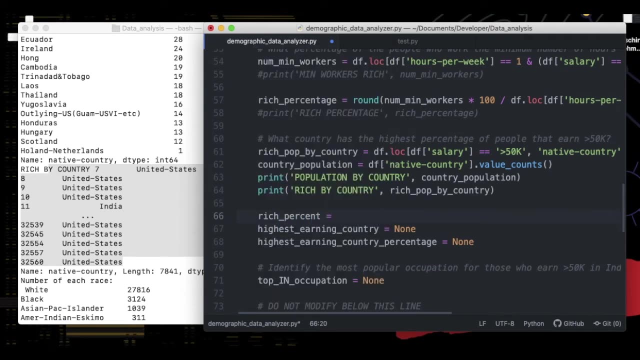 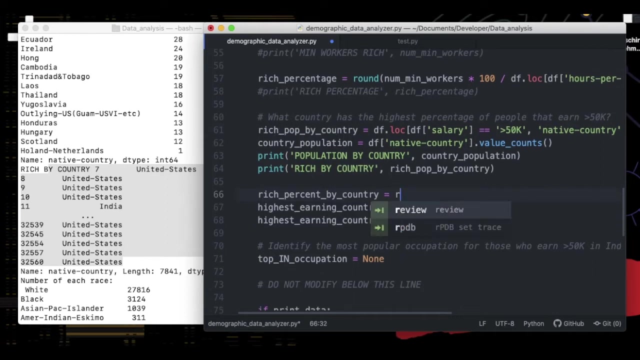 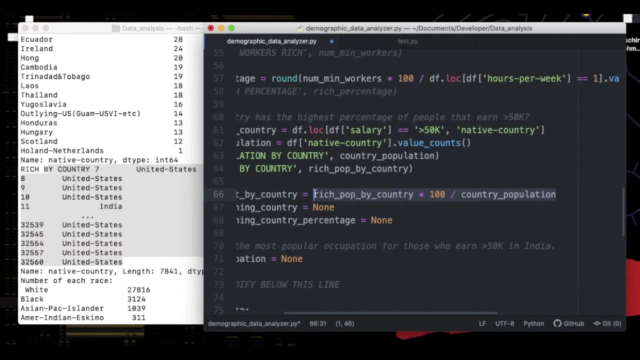 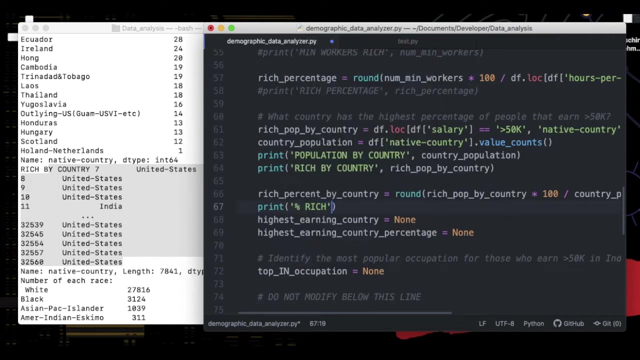 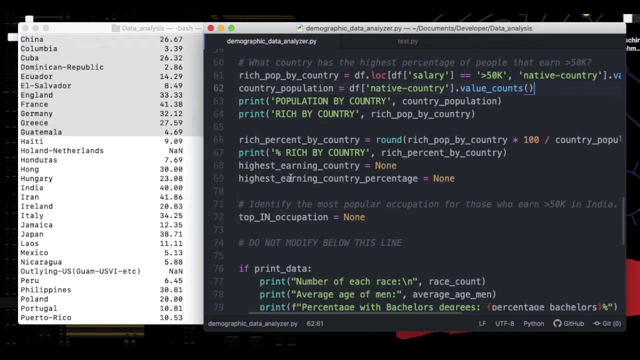 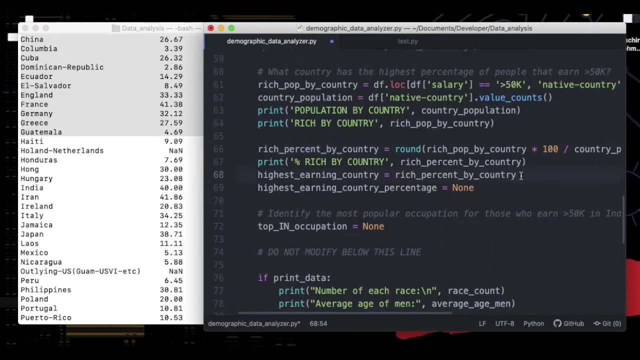 people by country. Thank you for watching. Now we have percent rich by country and then we want to find the top number, which is max. but here we want the name of the country. so we use function index max, which gives us the name of the country. 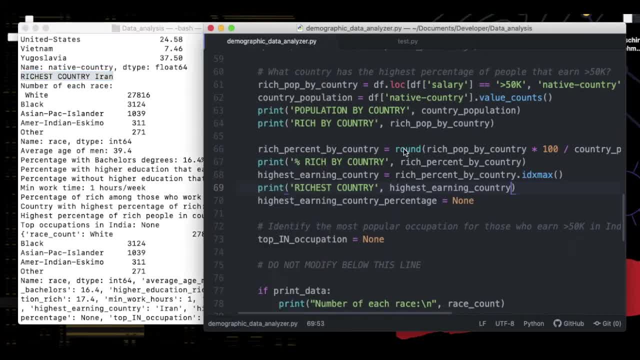 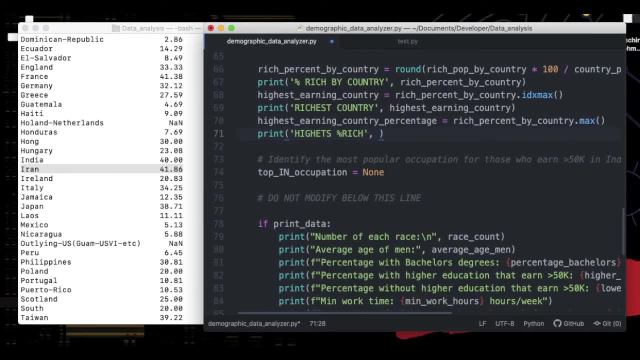 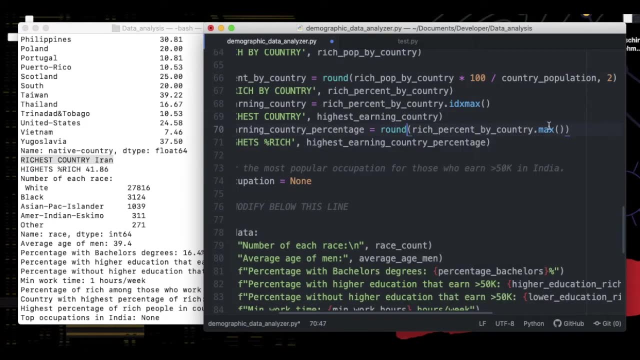 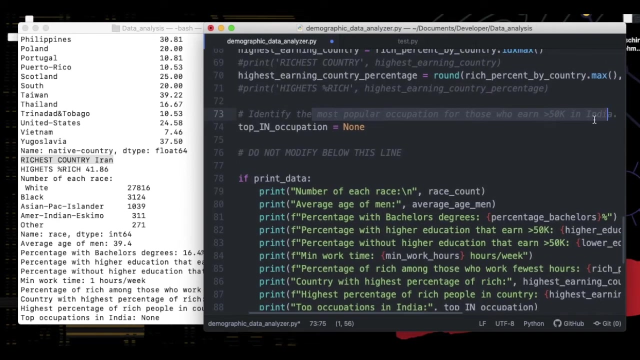 who has the highest percentage of rich people and similar. here we want max value now. so we use max function. that gives us the value of maximum number of selected column. and the last question is: to find a top occupation in India that rich people do. first select a country: India.